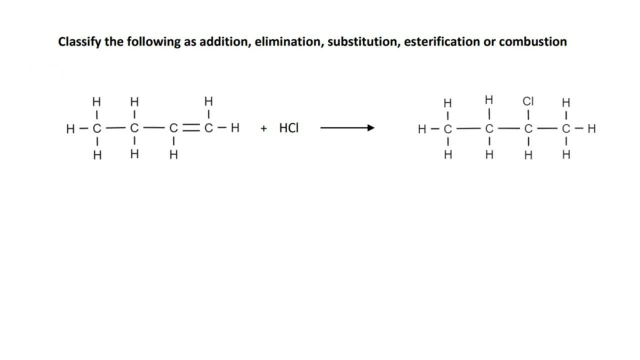 Classify the following reaction as addition, elimination, substitution, esterification or combustion. Thank you for watching. Each of those carbons now has three things. So that double bond that broke up can be, we can rather break it up and then rather add a little attachment or bond over here. So we can add a bond over there and we can add a bond over there. What then happens is that the H is going to go somewhere and the CO is going to go somewhere else. Now, according to Makhanikov's rule, this is where you have to. 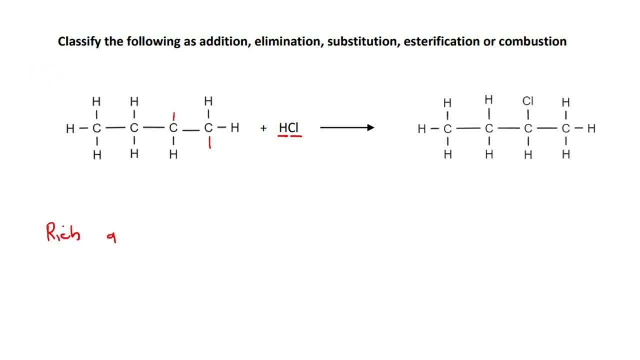 follow the riddle of the rich get richer and then the poor poorer get poorer. And remember that when we talk about this riddle, we are talking about hydrogen. Okay, And this part's not relevant. That's only when we do elimination. When you do addition, which is when you are adding molecules onto this molecule, that's called addition. You're adding things onto the molecule. 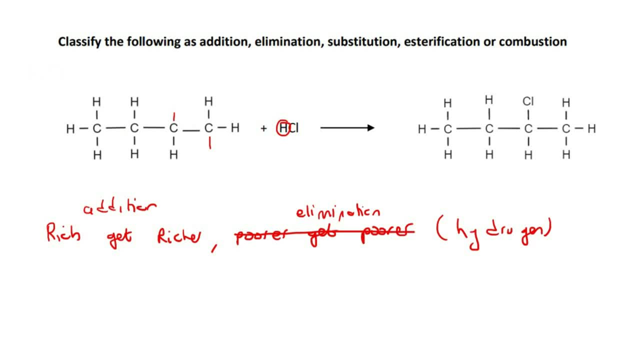 So this H is going to go to the carbon. It says that the rich get richer, So the carbon that already has the most hydrogen is going to get another hydrogen because the rich get richer. So he has a carbon with two hydrogens, whereas this carbon only has one. Some of you might be saying: yeah, but Kevin bro, listen up, This carbon has three. But we're not looking at that carbon, You're only allowed to look at the two carbons.